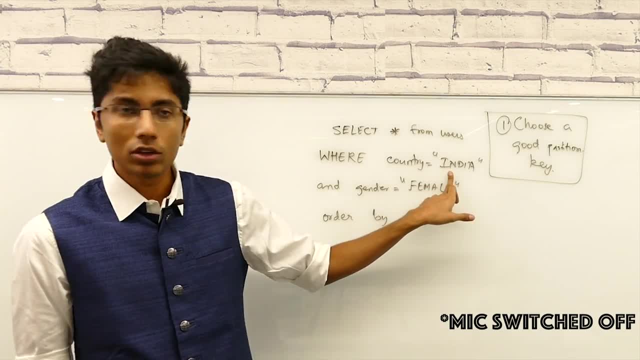 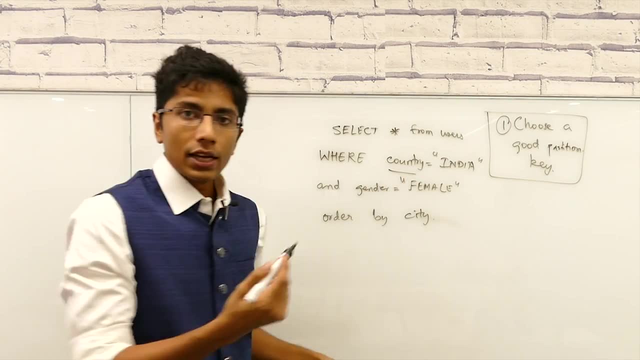 female, and I want it ordered by city. Let's say we have an index on this- the country, or we have the index on gender- both bad ideas. So let's say country: We get all the records of males and females who are in India. What you'll be then doing is you will be filtering through the record. 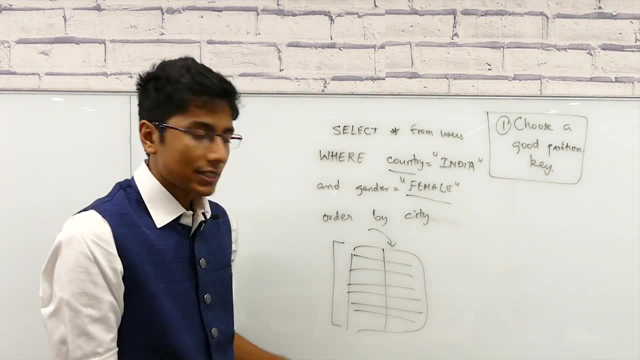 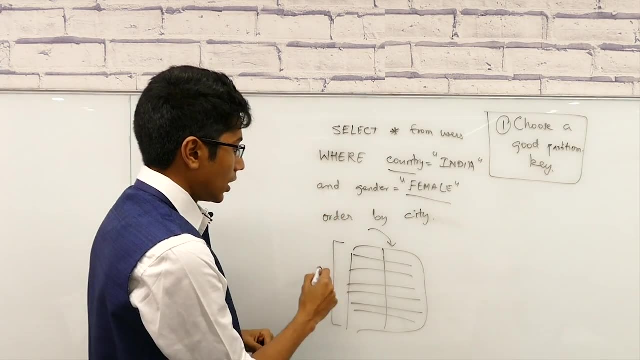 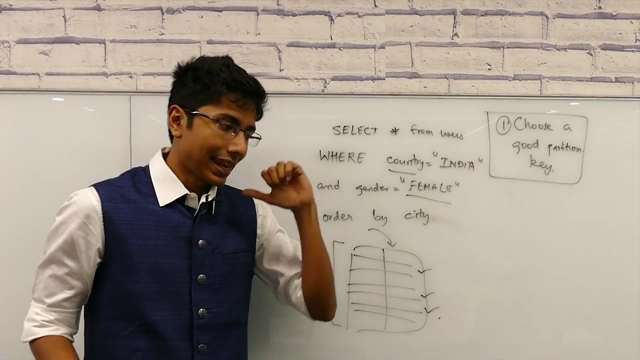 just choosing females. So the cost of this is equivalent to picking up all the people who are from India. Yeah, that's a big, big expense. Amongst this you filter out all of them who are female and then you actually sort them by city. So this is an expensive operation because it's order n in. 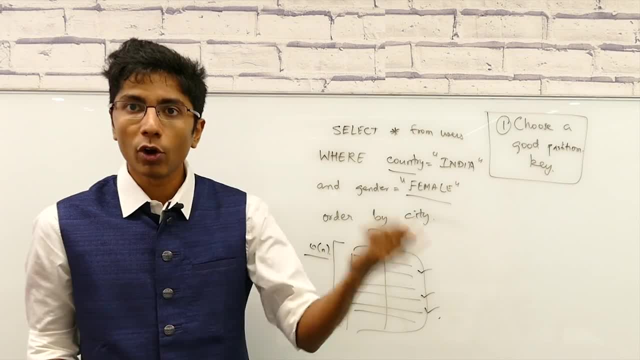 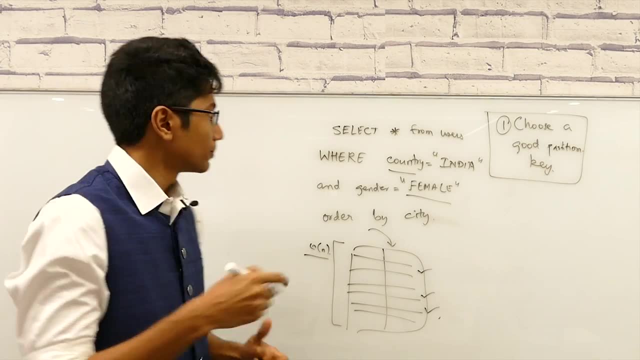 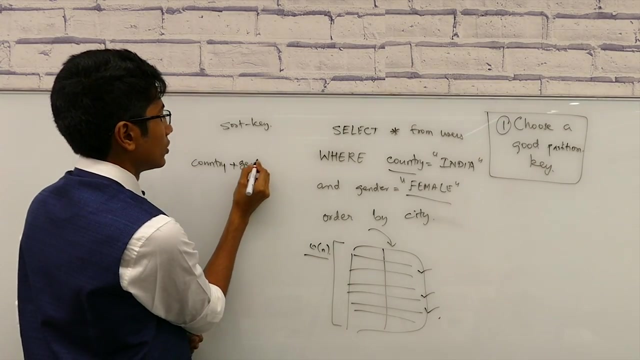 terms of the size of India, and then you sort that. so it's going to be order n login. Instead, what you can do is use an id. It's a sorting id. I'll call it the sort key. This is going to be defined by country plus gender. 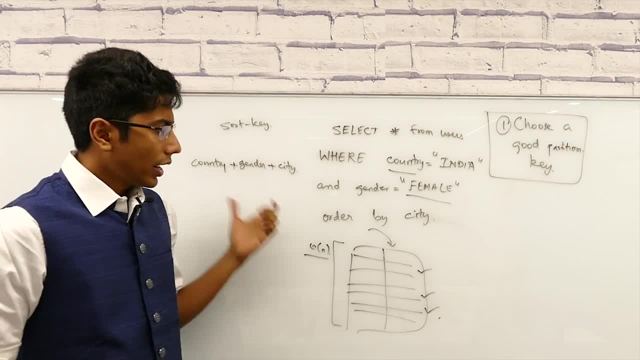 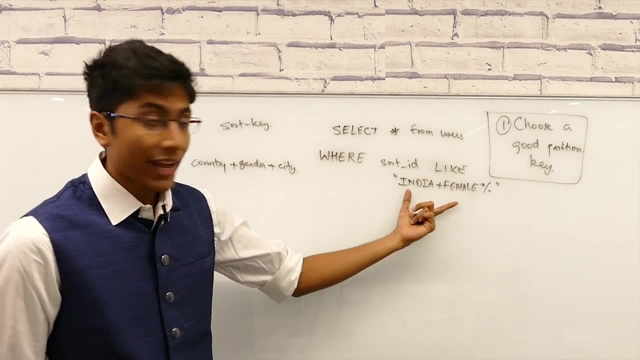 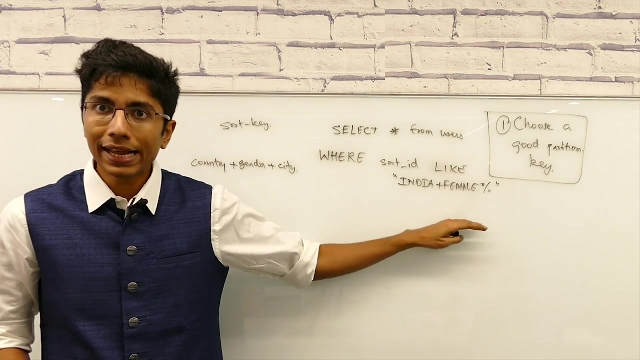 plus city. How is this better? Well, if you have that sort id, now the where turns into the sort id running on a regex of India plus, female plus, and that's it. Now, of course, there's an index on this. So what's going to end up happening is that you will just 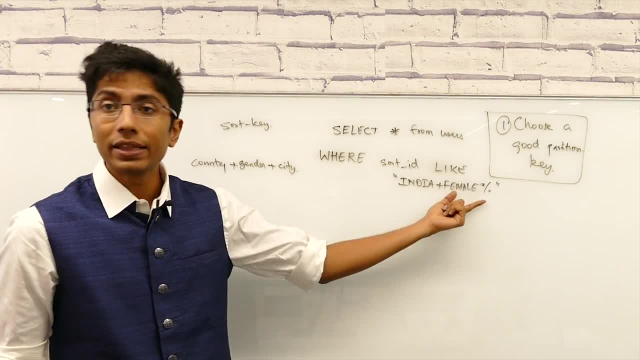 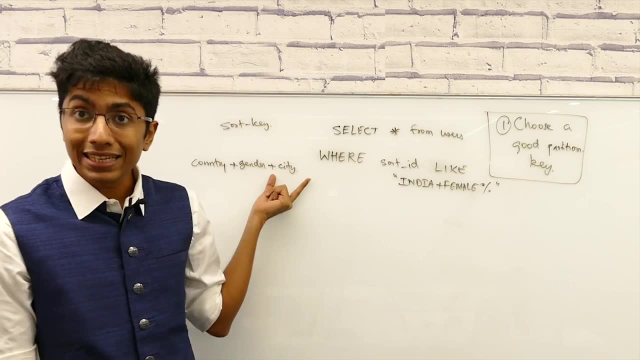 run through all the records where India plus female will be there and because of the binary search thing you're going to be landing on a nice range in which India and female are there. If you have it sorted on city already, you can just pull out all the records and solve that to the user. This gives you huge savings. So the main difference seems to be that normalization is strongly discouraged in NoSQL databases. I mean, doesn't exist really. You shouldn't be normalizing tables if you have got the NoSQL. Yes, you can't avoid the redundancy, You have to keep. the data together and you can't avoid the redundancy. You can't avoid the redundancy. You can't avoid the data together and you can't avoid the redundancy. You have to keep the data together and you can't avoid the redundancy. You have to keep the data together and you can't avoid the redundancy. And if you're 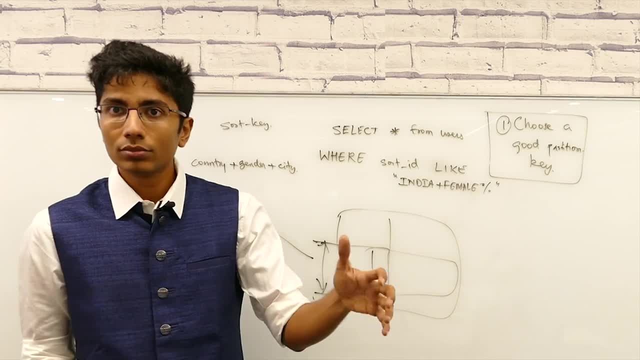 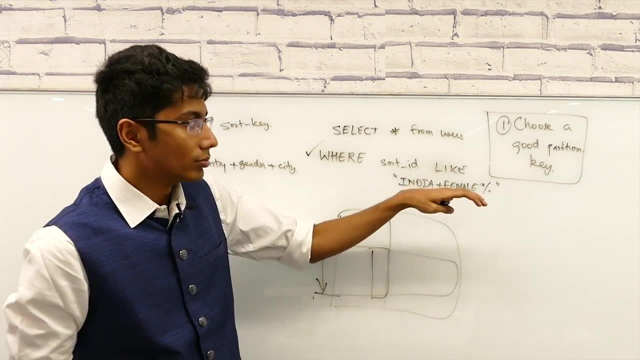 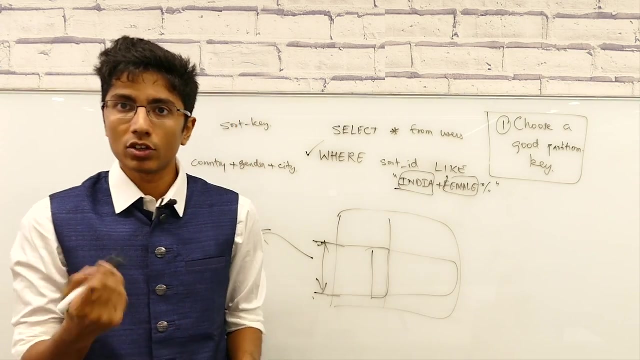 looking for indexing, it seems like multi-column keys are very natural in NoSQL databases. So this is the way you index in a NoSQL database. In normal databases you will be having India separate and female separate, and so on, so forth, because of normalization. 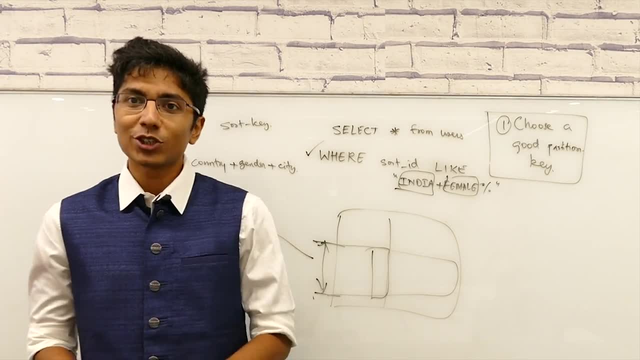 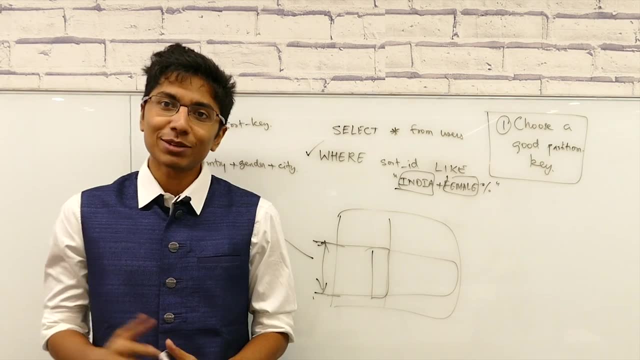 So that's it for indexing databases. If you have any doubts or suggestions for this, you can leave them in the comments below. If you like the video, then make sure to hit the like button, and if you want notifications for further videos like this, hit the subscribe button. I'll see you next time. 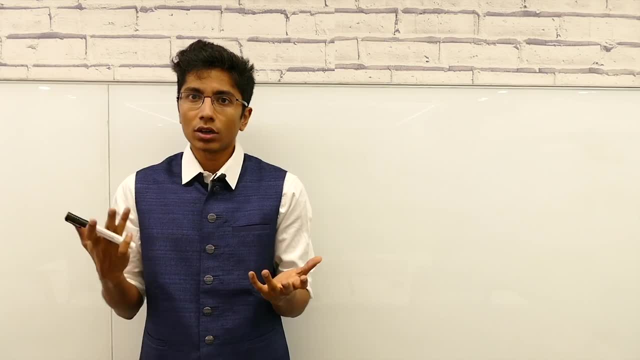 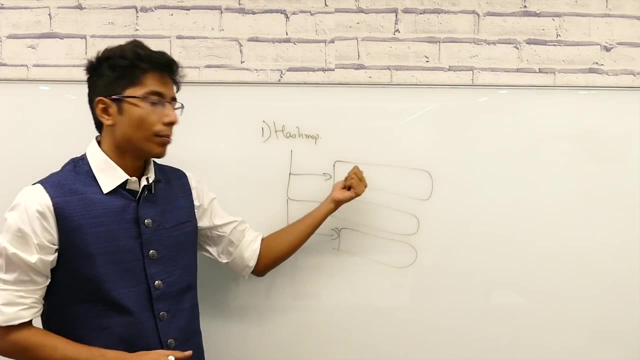 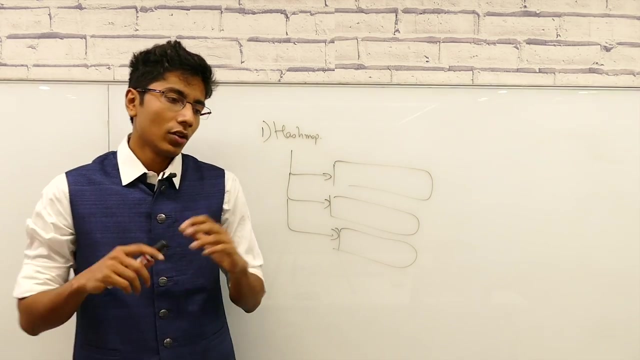 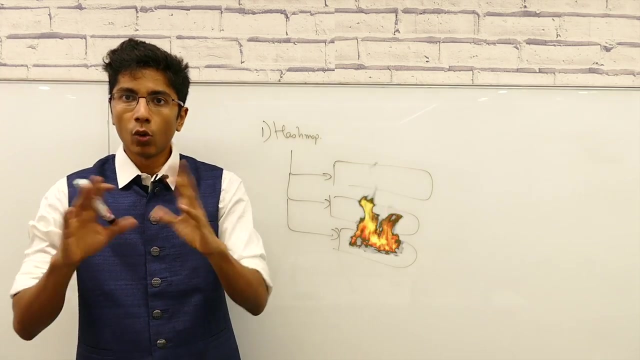 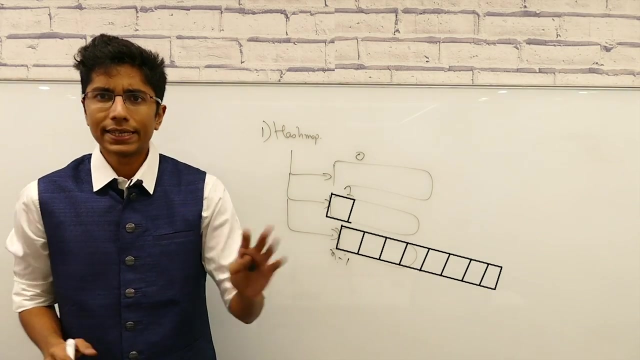 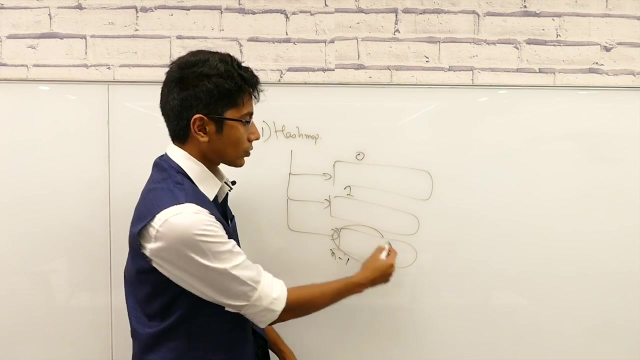 Thanks for watching. This is the worst case in a hash map. So the next thing that you can do- which is exactly what happened in the interview- is that I'll make a hash map out of these two with a different key. So let's say the object was name, age, gender, so on and so forth. So 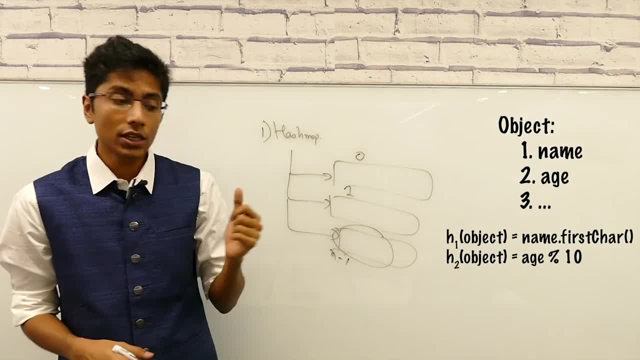 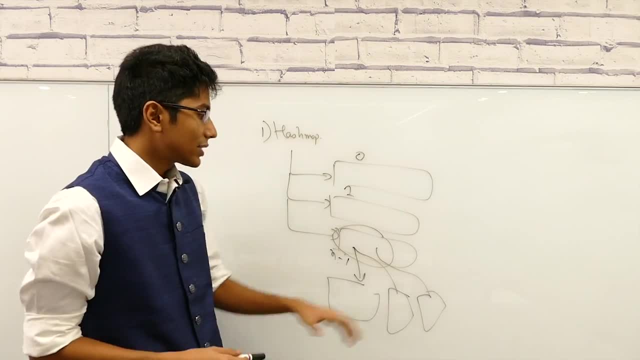 the name would be on. the first would be defining the first hash map. that would be the first key. The age would define the next hash map and your assumption is that they're going to be different at some point. What if this hash map is also completely skewed? What if the first bucket 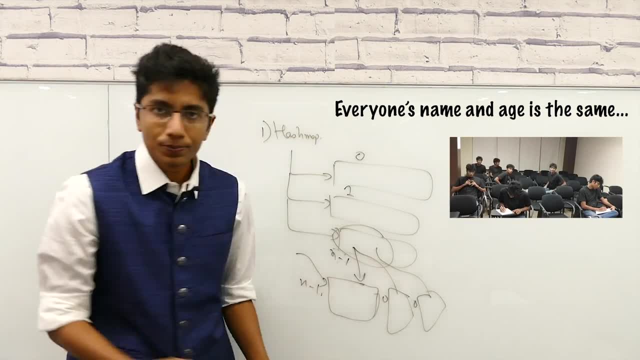 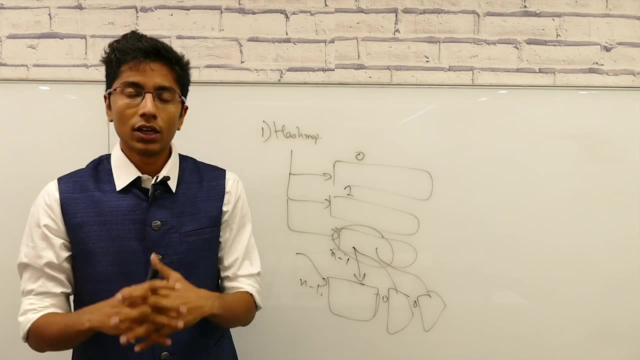 has all the elements n-1 and the other ones have 0 and 0?. I have never seen scenarios where a three-layer hash map or a four-layer hash map is not giving you efficient query patterns. At that time you have to actually start blaming the developer who thought about the stupid. 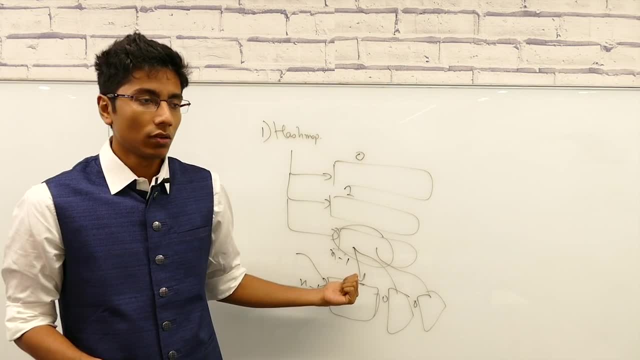 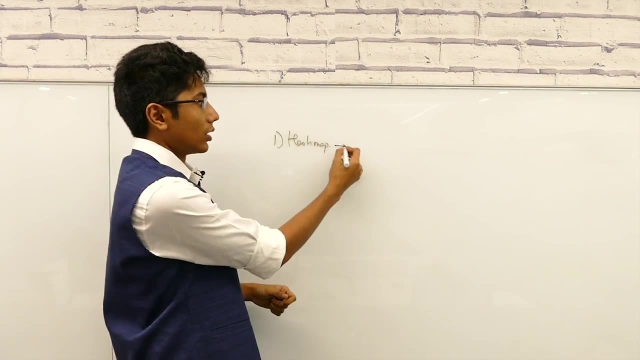 key over here and the stupid key over here, But I guess you can't say that in an interview. What you can do, though, in this hash map solution, is augment it with another data structure, which is binary search tree, But a binary search tree has the problem. 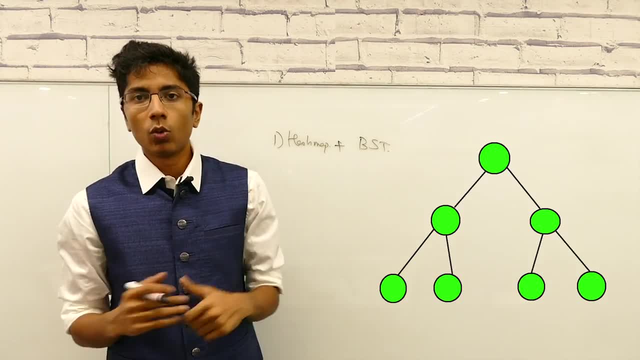 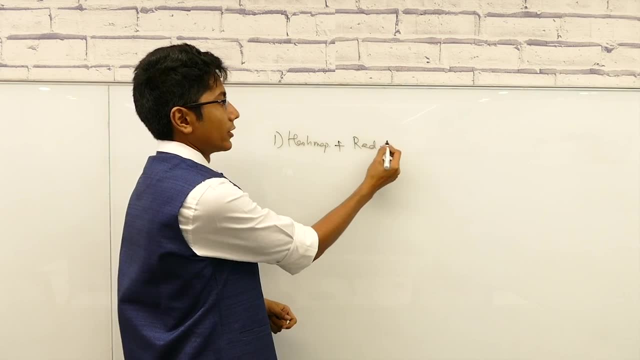 that it can get very skewed. So what we are going to do is we are going to have a height balance binary search tree, which is basically a. I mean, there's multiple limitations, but we can have a red black tree here, And so the queries are really efficient. The queries are log in. 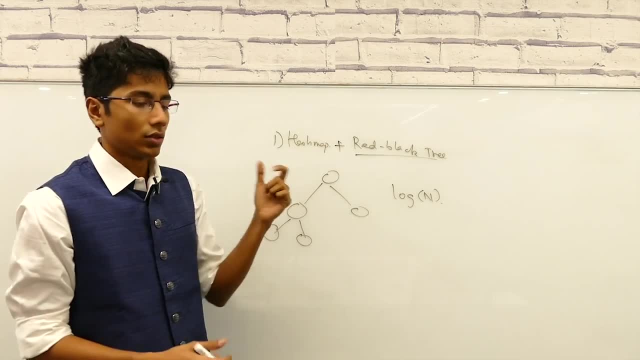 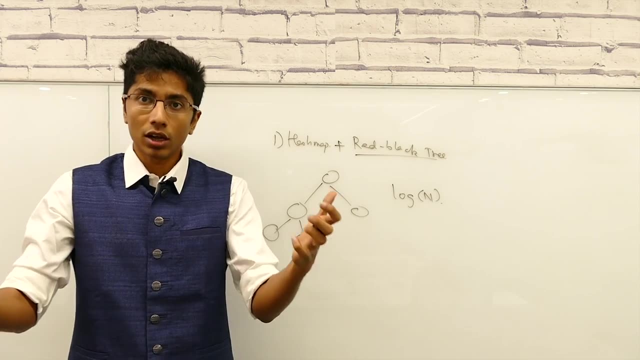 So in the best case, amortize- you're going to get order one query time in the hash map. And in the worst case, because once you went down to, let's say, three levels and you see that there's still a ton of entries, there's a threshold value. So if the threshold is, let's say, 100, 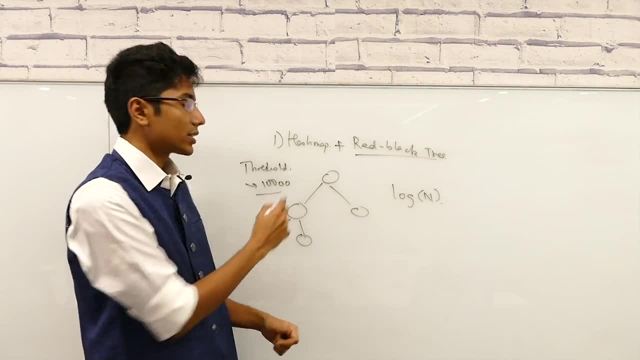 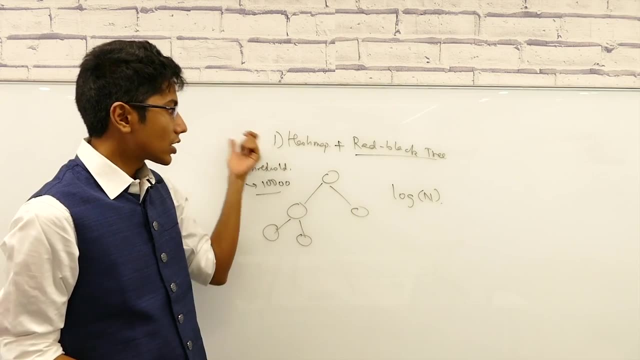 elements come in, then you don't do linear search anymore. Or let's say, 10,000 elements come in, you don't do linear search anymore. You will convert that data into a red black tree And then whenever there's a query on that bucket you can just respond in order: log n time.